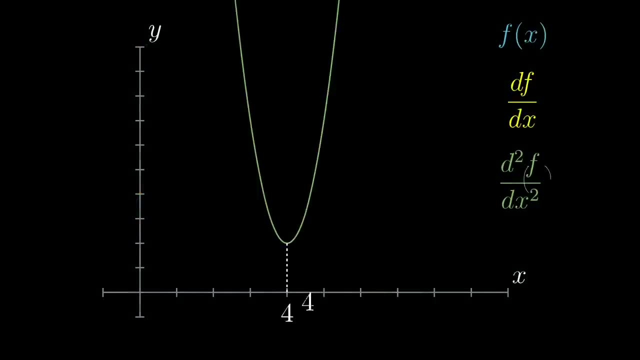 For example, a graph like this one has a very positive second derivative at the point 4, since the slope is rapidly increasing around that point, Whereas a graph like this one still has a positive second derivative at the same point, but it's smaller. I mean the slope only increases slowly At points where there's not. 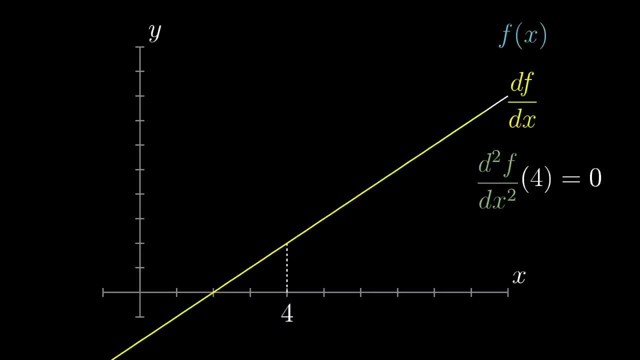 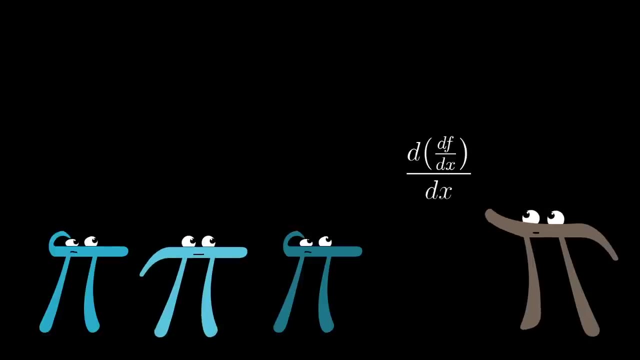 really any curvature. the second derivative is just zero. As far as notation goes, you could try writing it like this, indicating that the second derivative is positive, But if you're writing some small change to the derivative function divided by some small change to 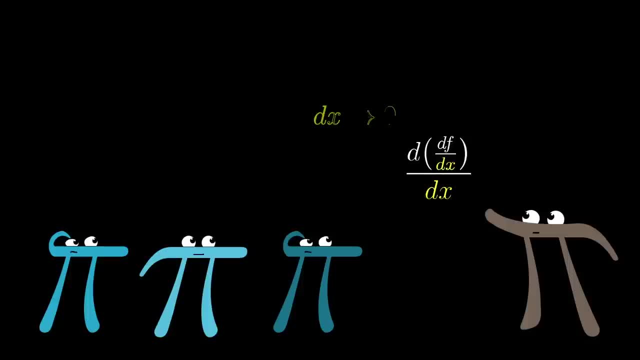 x, where, as always, the use of the letter d suggests that what you really want to consider is what this ratio approaches as dx approaches 0.. That's pretty awkward and clunky, So the standard is to abbreviate this as: d squared f divided by dx squared And. 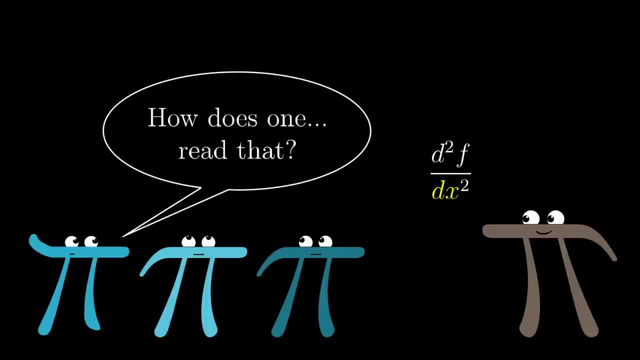 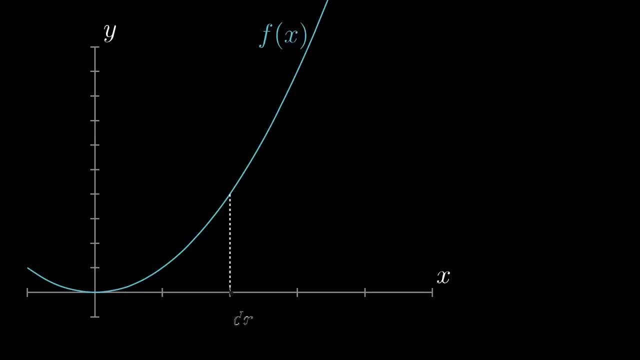 even though it's not terribly important for getting an intuition for the second derivative derivative, I think it might be worth showing you how you can read this notation. To start off, think of some input to your function and then take two small steps to the right, each one with 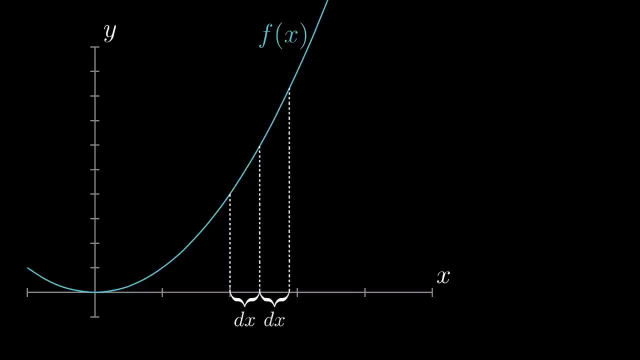 the size of dx. I'm choosing rather big steps here so that we'll be able to see what's going on, but in principle, keep in the back of your mind that dx should be rather tiny. The first step causes some change to the function, which I'll call df1, and the second step causes 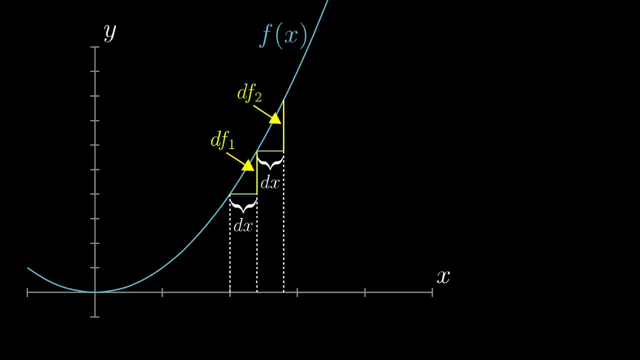 some similar but possibly slightly different change, which I'll call df2.. The difference between these changes, the change in how the function changes, is what we'll call ddf. You should think of this as really small, typically proportional to the size of dx. 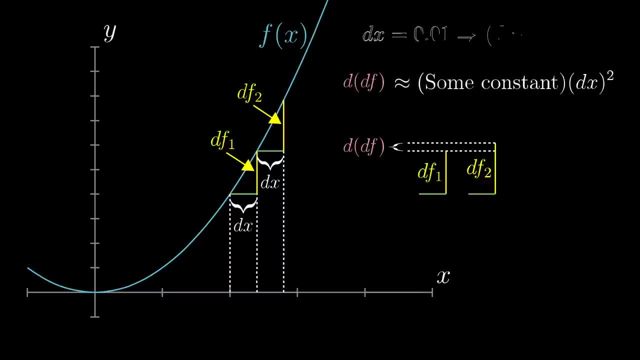 squared. So if, for example, you substituted in 0.01 for dx, you would expect this ddf to be about proportional to 0.01.. And the second derivative is the size of this change to the change divided by the size of.